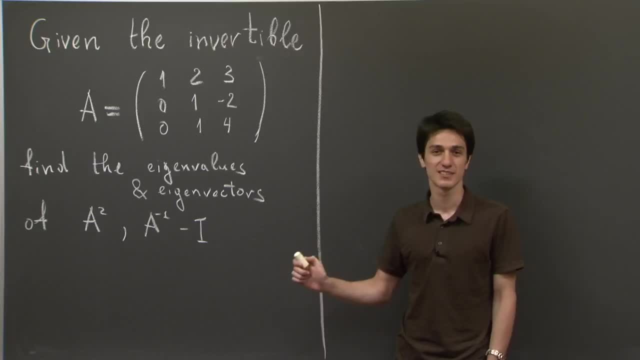 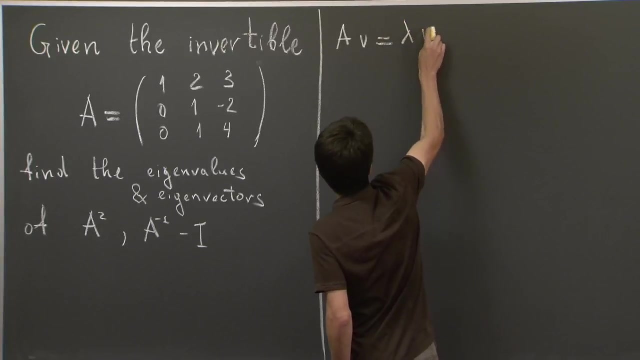 give you a few moments to think of your own line of attack and then you'll see mine Hi again. OK, so the observation that makes our life really easy is the following one: So say V is an eigenvector with associated eigenvalue lambda to A, the matrix A. Then if we hit, 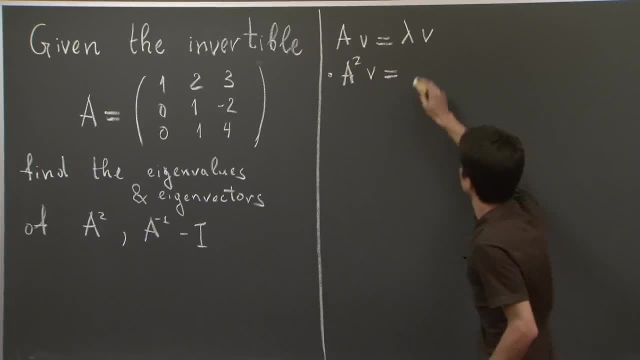 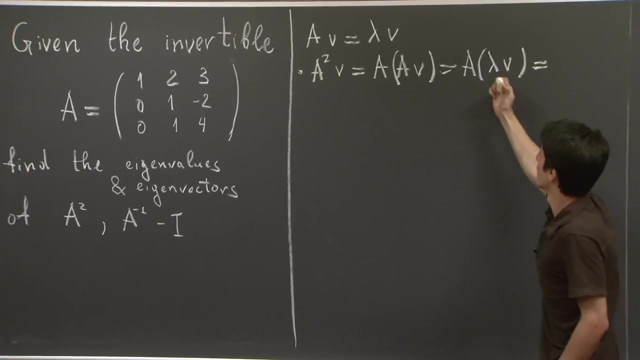 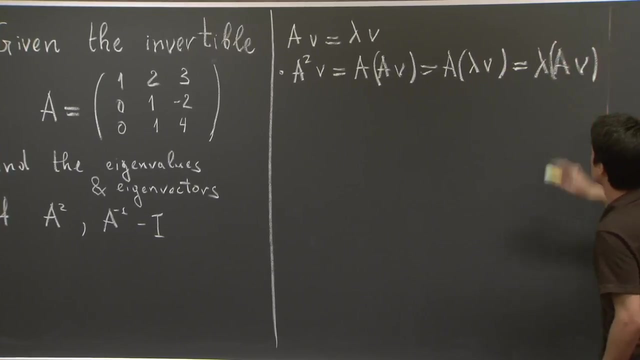 V with A squared. well, this we can write it as A times A V, But A V is lambda V, right? So we have A lambda V. Lambda is a scale, So we can move it in front and we get lambda A V. And lambda A V is when we plug in A V. 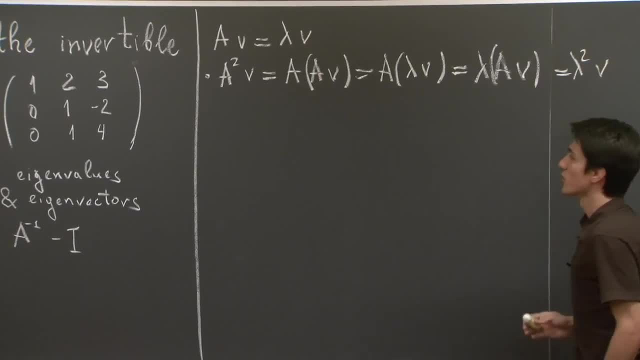 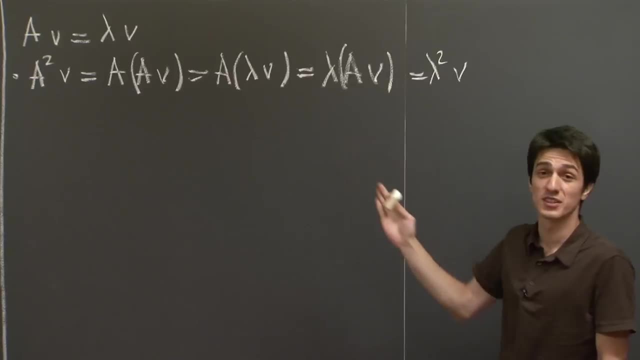 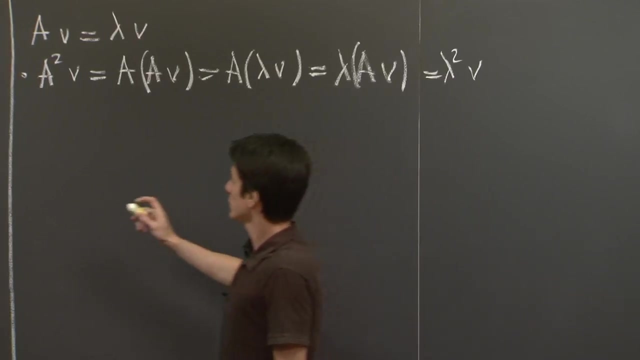 lambda V is just lambda squared V. So what we've found out is that if V is an eigenvector for A, then it's also an eigenvector for A squared, just that the eigenvalue is the eigenvalue squared. Similarly. 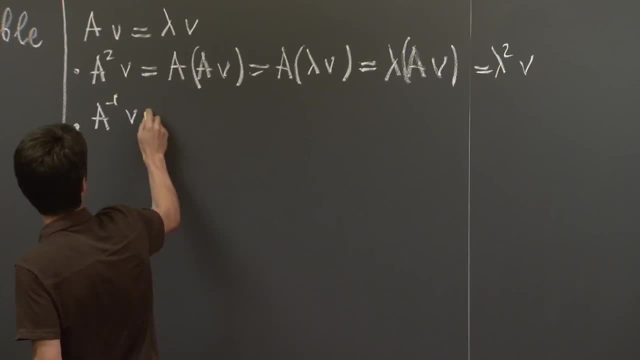 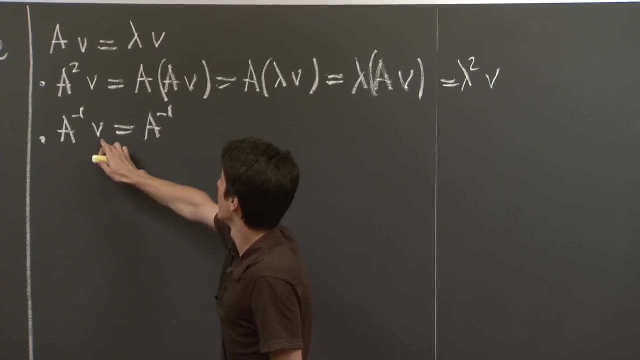 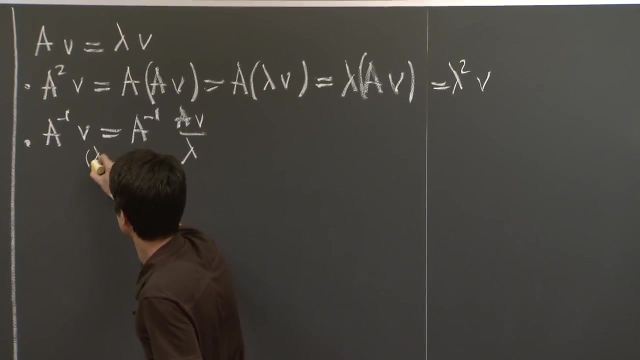 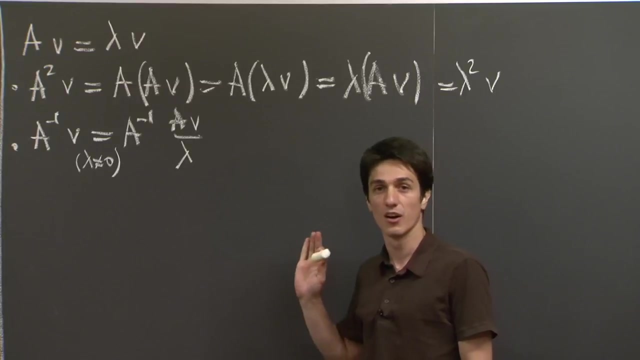 if we hit A inverse, if we hit V with A inverse. so in this case, we can write V as A V over lambda, given that, of course, lambda is non-zero, But the eigenvalues of an invertible matrix are always non-zero, which is an exercise you should do yourself. 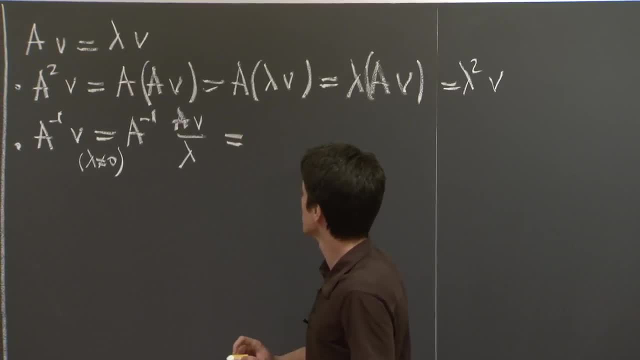 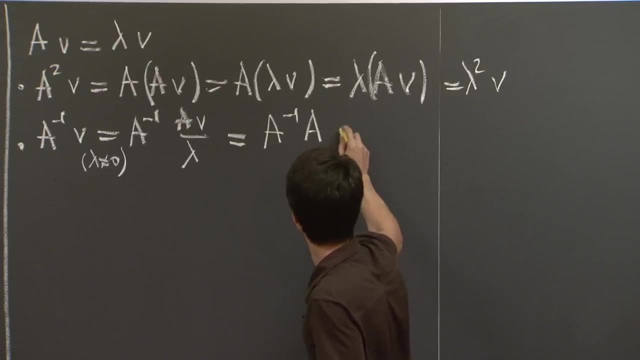 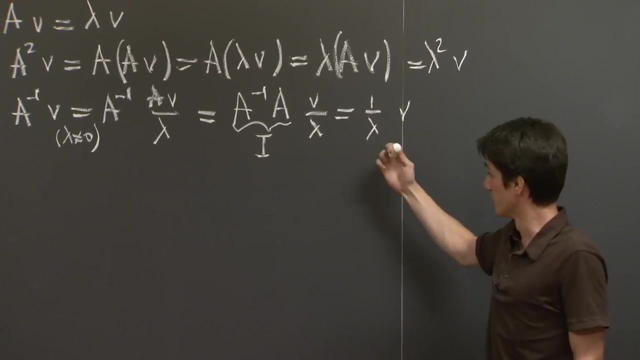 So if we just then take out the A and combine it with A inverse, this is the identity, And so we get 1 over lambda V. So V is also an eigenvector for A inverse with eigenvalue, the reciprocal of lambda. 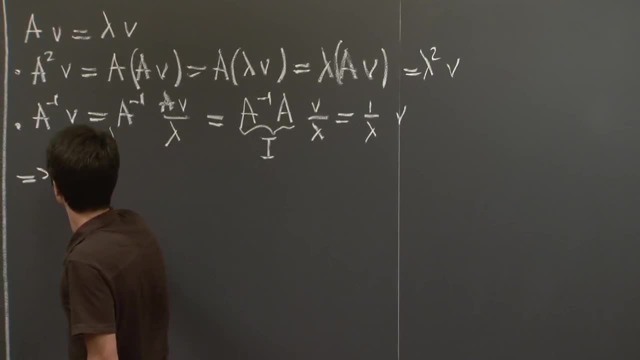 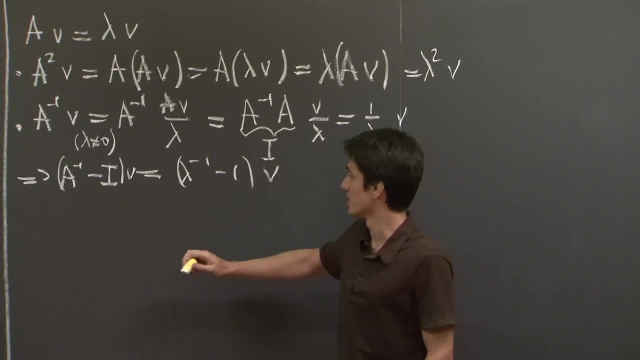 OK, And from here of course. OK. So A inverse minus the identity is lambda inverse minus 1 V. So the eigenvalue associated with the eigenvalue of A inverse minus the identity is 1 over lambda minus 1.. OK, 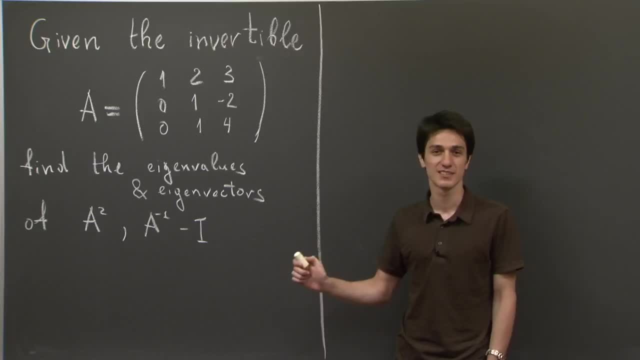 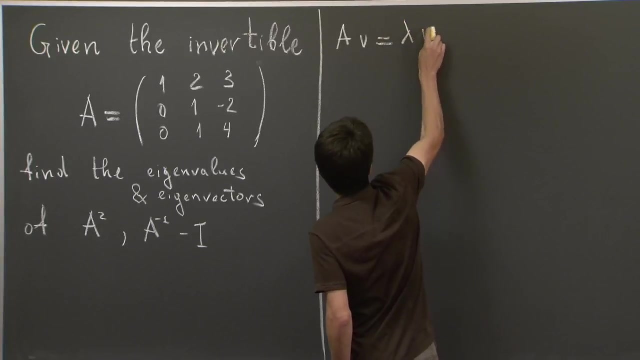 give you a few moments to think of your own line of attack and then you'll see mine Hi again. OK, so the observation that makes our life really easy is the following one: So say V is an eigenvector with associated eigenvalue lambda to A, the matrix A. Then if we hit, 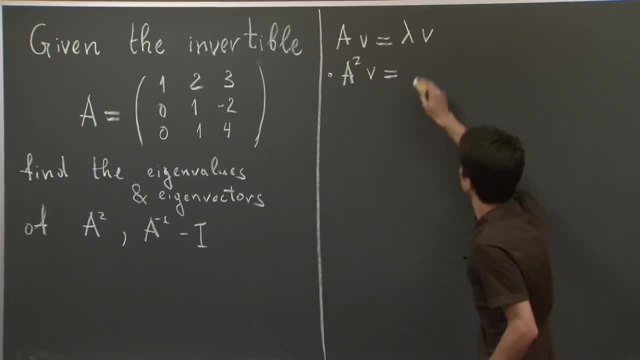 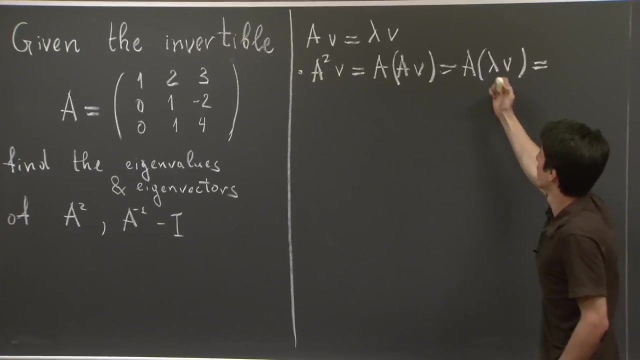 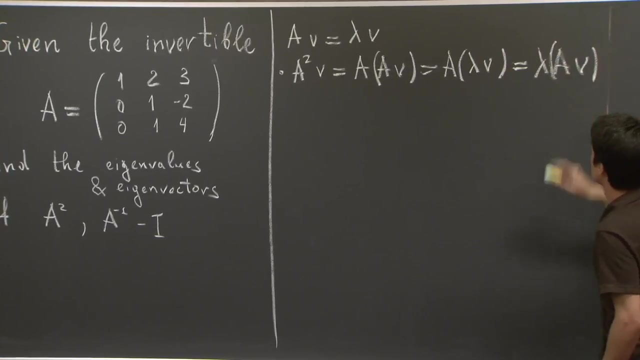 V with A squared. well, this we can write it as A times A V, But A V is lambda V, right? So we have A lambda V. Lambda is a scale, So we can move it in front And we get lambda A V. And lambda A V is when we plug in A. 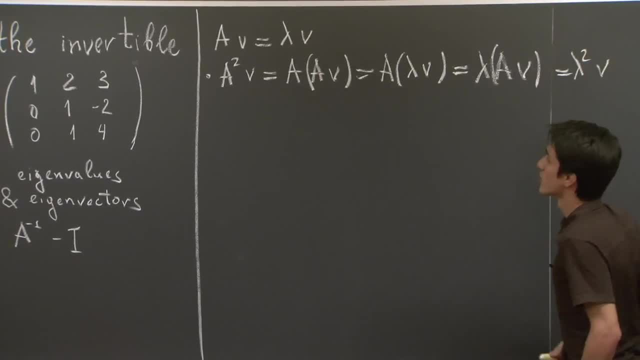 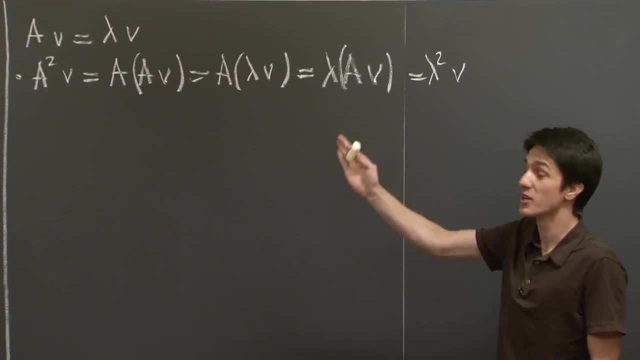 V lambda. V is just lambda squared V. So what we've found out is that if V is an eigenvector for A, then it's also an eigenvector for A squared, just that the eigenvalue is the eigenvalue squared. 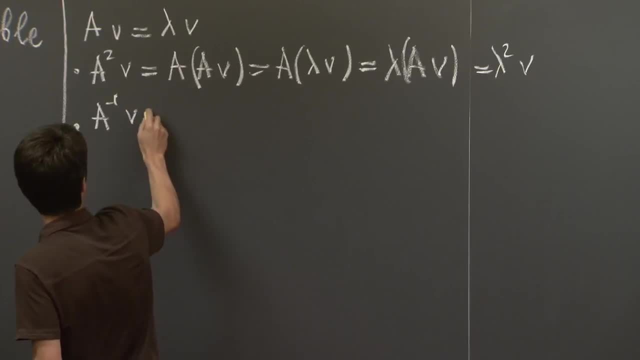 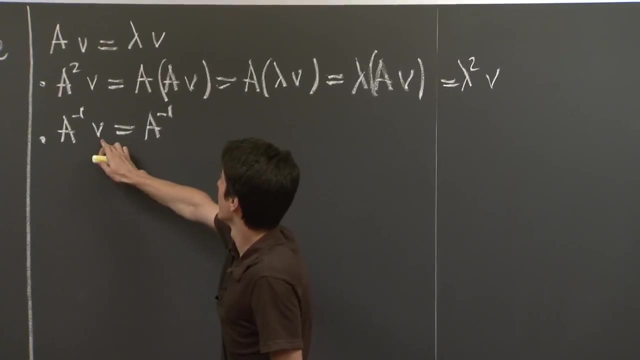 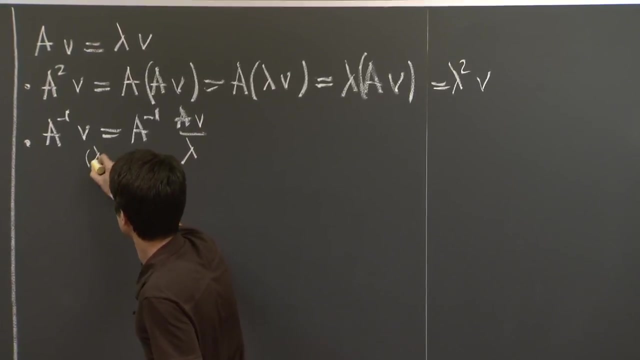 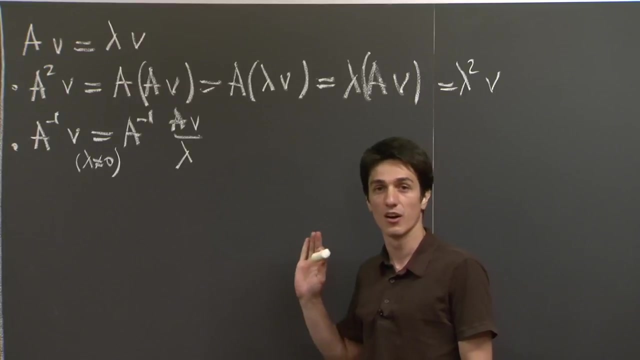 So if we hit A inverse, if we hit V with A inverse, so in this case we can write V as A V over lambda, given that, of course, lambda is non-zero, But the eigenvalues of an invertible matrix are always non-zero, which is an exercise you should do. 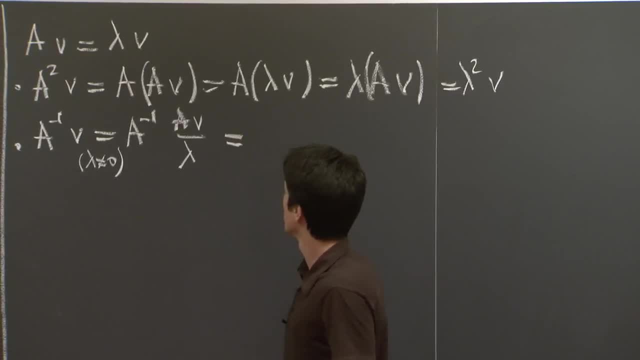 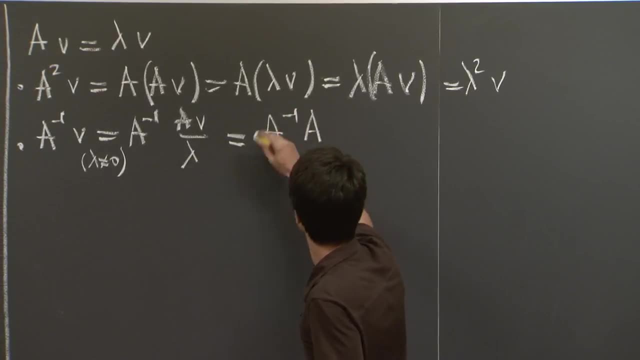 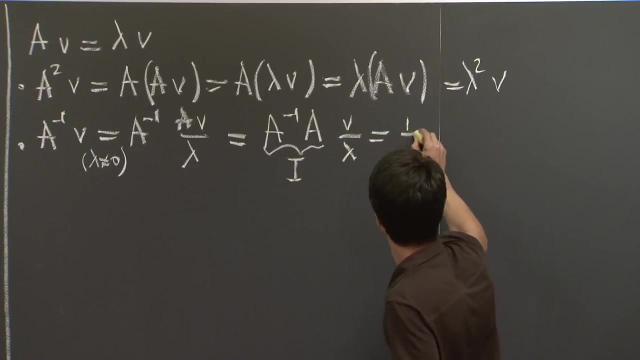 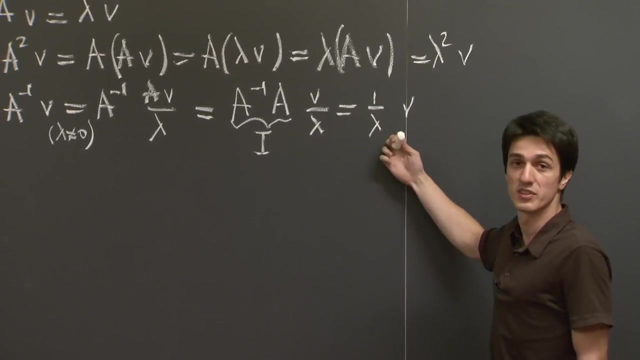 yourself OK. So if we just then take out the A and combine it with A inverse, this is the identity, And so we get 1 over lambda V. So V is also an eigenvector for A inverse with eigenvalue, the reciprocal of lambda. 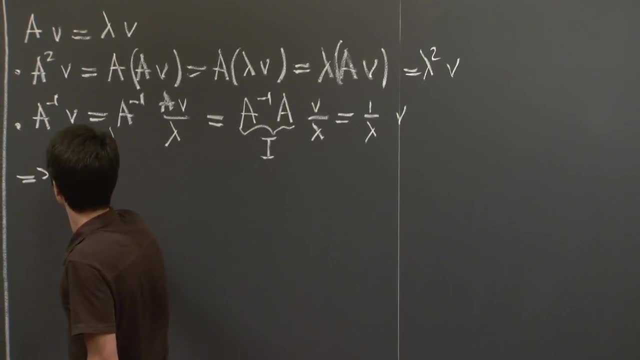 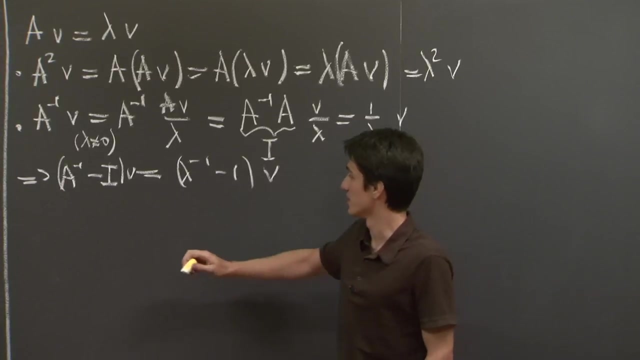 OK, And from here of course. So this is A inverse minus the identity, is lambda inverse minus 1 V. So the eigenvalue associated with, so the eigenvalue of A inverse minus the identity is 1 over lambda minus 1.. 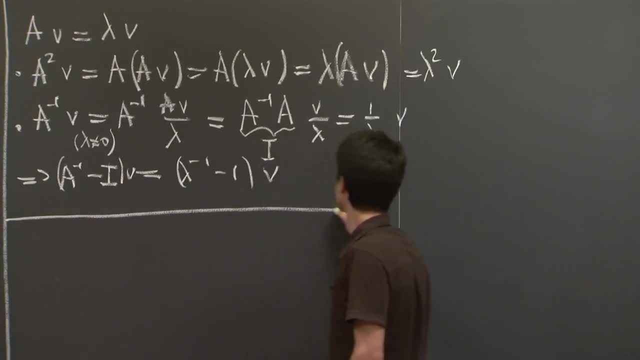 OK, So what we've figured out is we just need to find the A inverse minus the identity. So we just need to find the eigenvalues and eigenvectors of A, And then we have a way of finding what the eigenvalues and eigenvectors of those combinations. 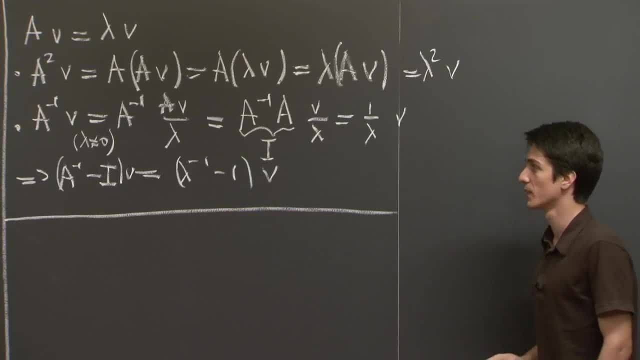 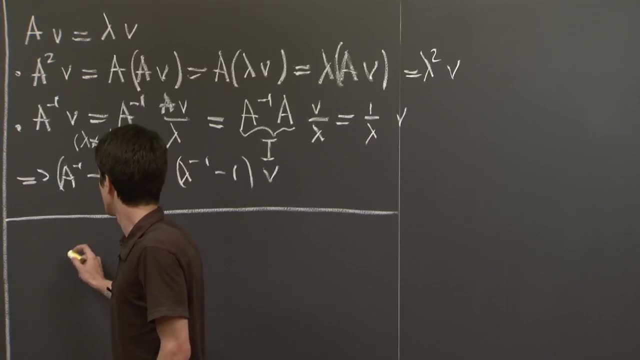 well, A squared and A inverse minus the identity will be OK. So how do we find the eigenvalues? Well, what does it mean for lambda to be an eigenvalue of A? It means that the matrix A minus lambda, Lambda, the identity, is singular. 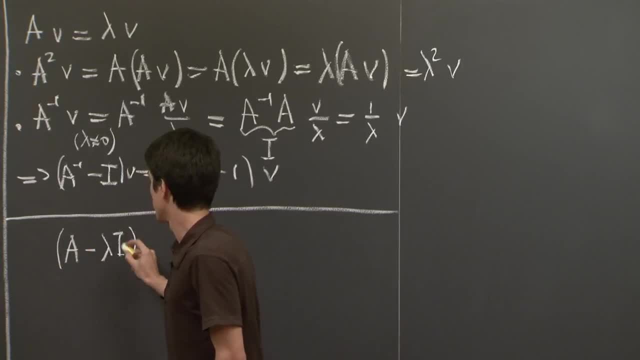 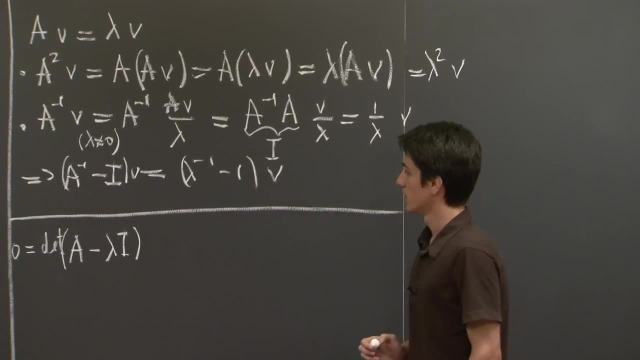 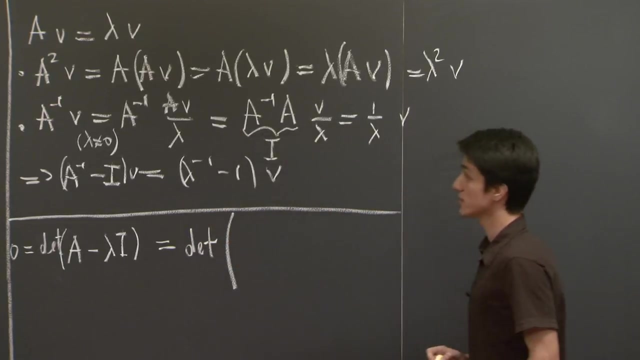 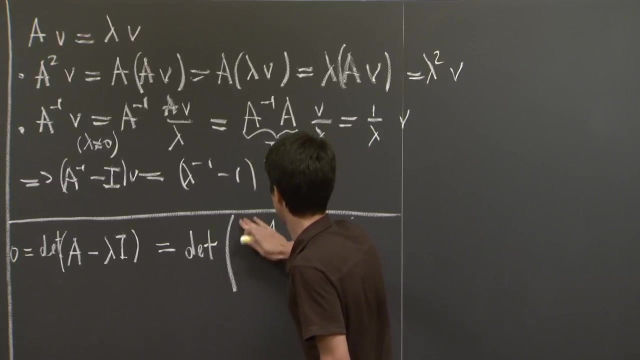 Which is precisely the case when its determinant is 0.. OK, So we have. we need to solve the following equation: lambda minus 1, 2, 3.. Oh sorry, 1 minus lambda, OK, 2, 3.. 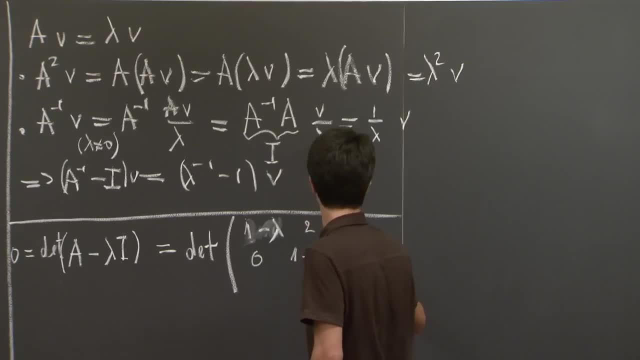 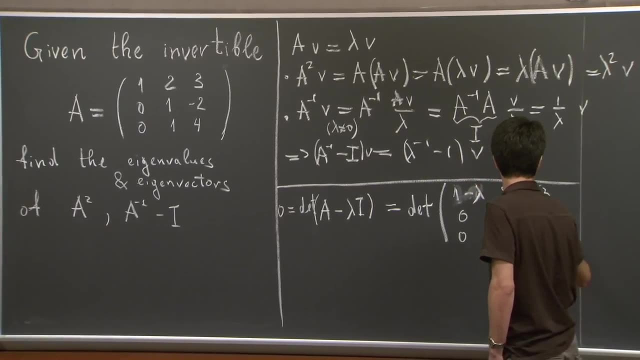 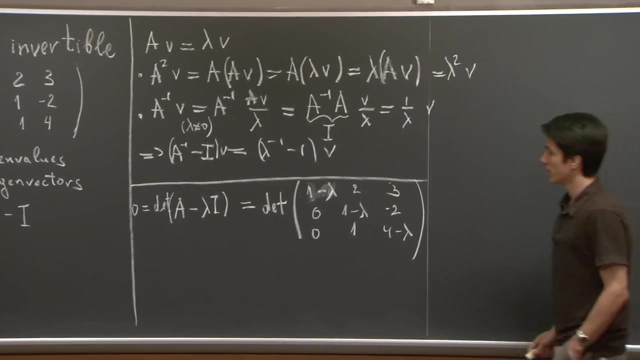 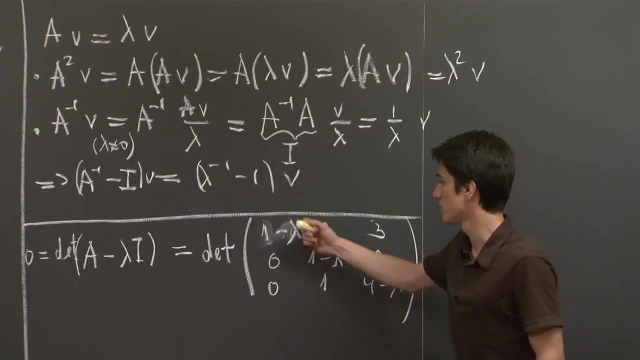 0, 1 minus lambda 2, negative 2.. And 0, 1, 4 minus lambda. OK, So it's fairly obvious which column we should use to expand this determinant. We should use the first column because we have only one non-zero entry. 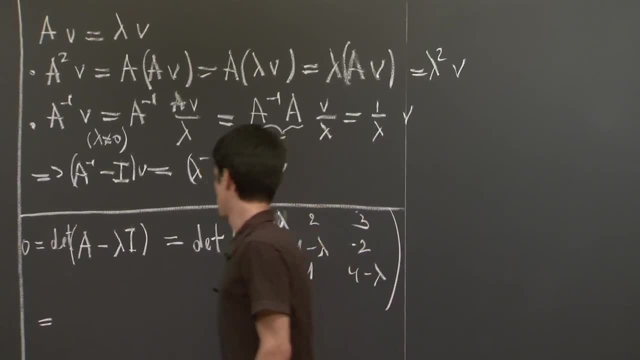 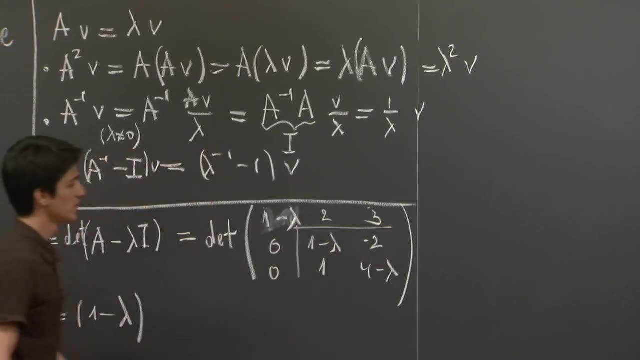 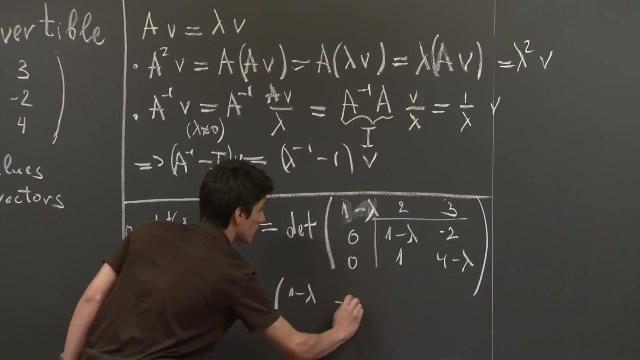 And so this is equal to 1 minus lambda times the determinant of the 2 by 2 matrix: 1 minus lambda, negative 2, 1, 4 minus lambda, Which is? I'm going to take the first column. 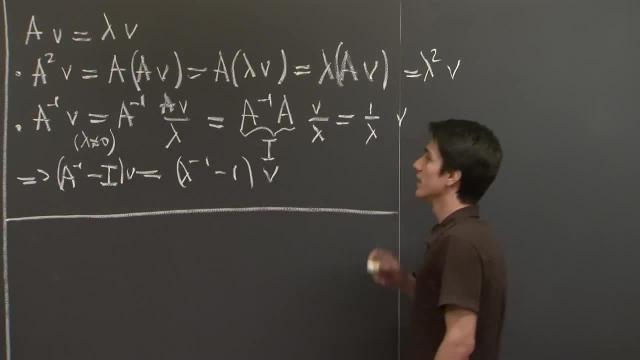 So what we've figured out is we just need to find the eigenvalues and eigenvectors of A, And then we have a way of finding what the eigenvalues and eigenvectors of those combinations. Well, A squared and A inverse minus the identity will be. 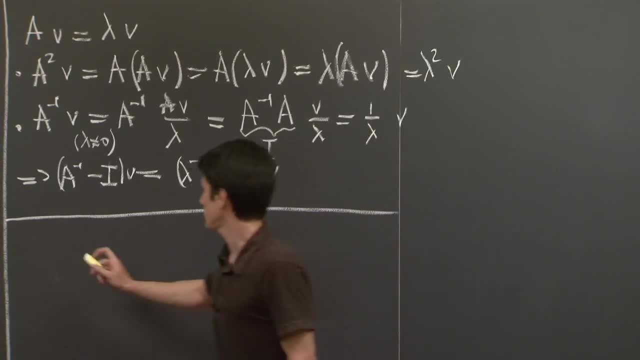 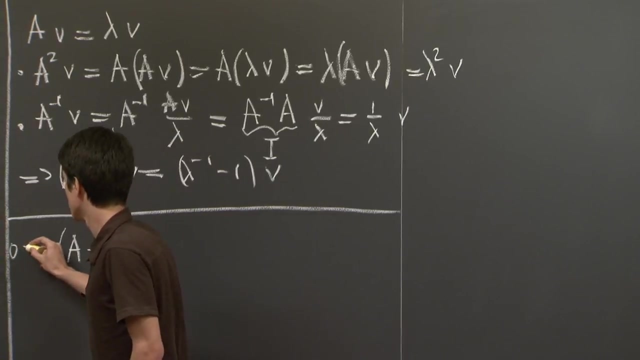 OK, So how do we find the eigenvalues? Well, what does it mean for lambda to be an eigenvalue of A? It means that the matrix A minus A inverse minus 1 V is lambda. The identity is singular, Which is precisely the case when its determinant is 0. 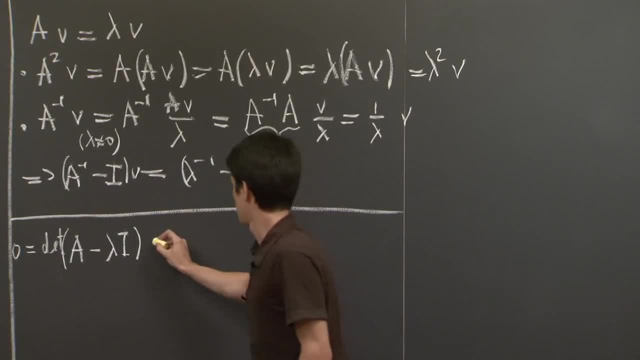 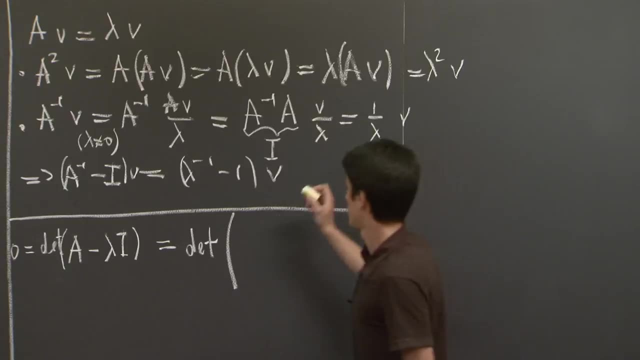 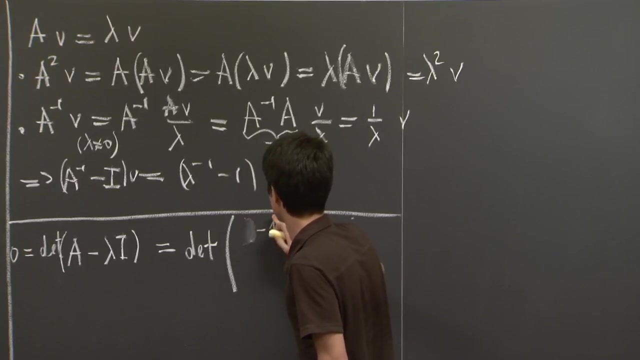 OK, So we need to solve the following equation: lambda minus 1, 2, 3.. Oh sorry, 1 minus lambda 2, 3.. 0, 1 minus lambda 2, negative 2.. 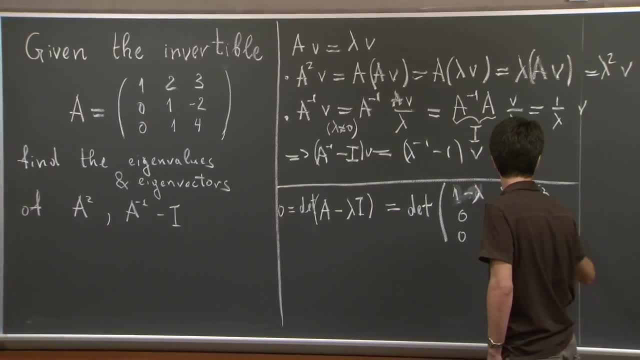 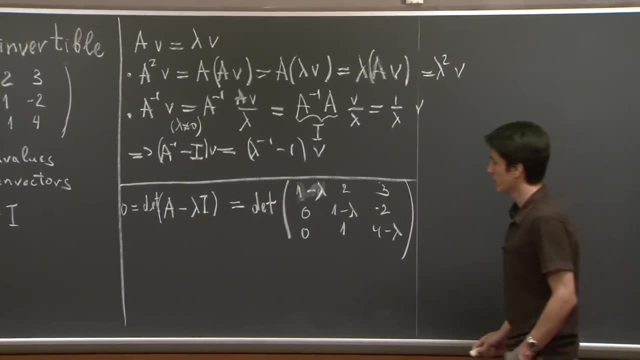 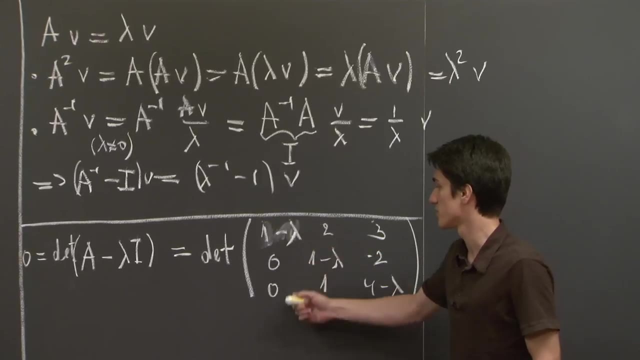 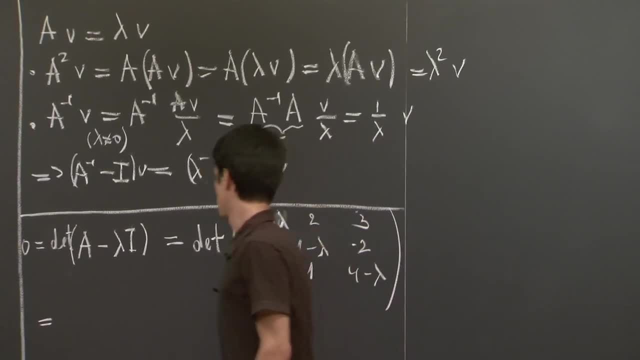 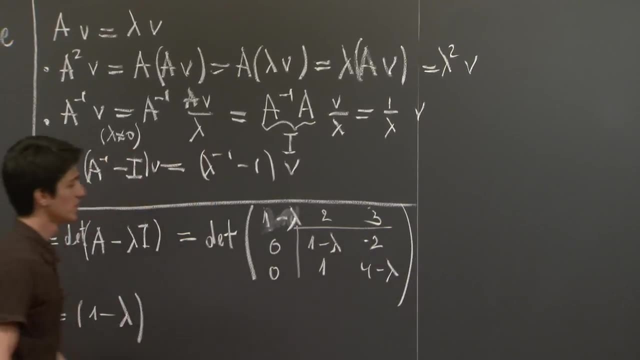 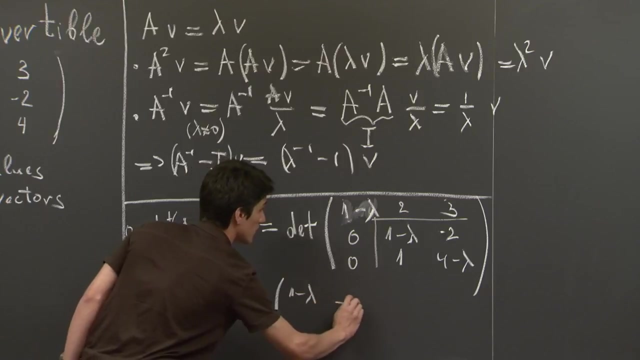 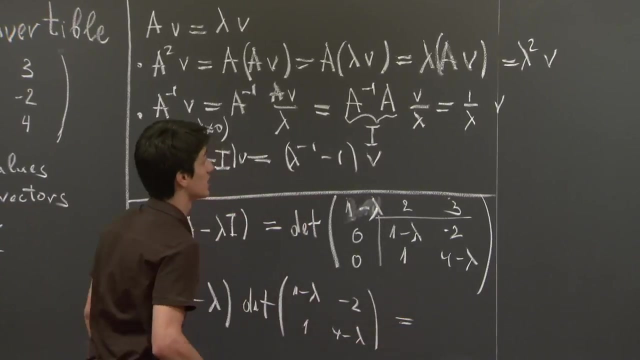 And so this is equal to 1 minus lambda times the determinant of the 2 by 2 matrix: 1 minus lambda, negative 2, 1, 4 minus lambda, which is- I'm going to take the computation up here. 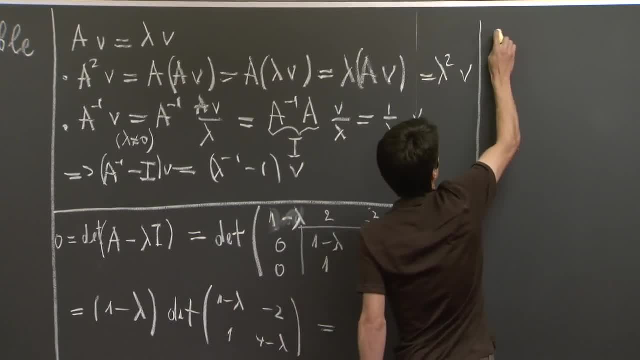 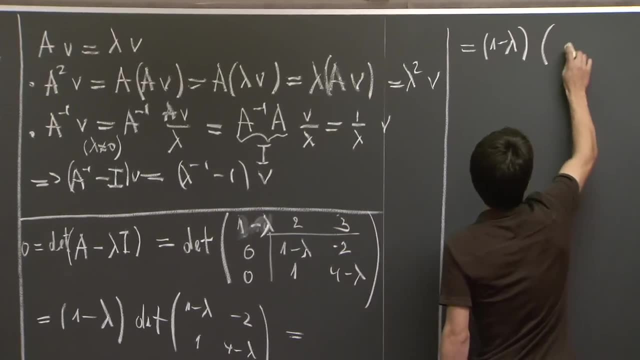 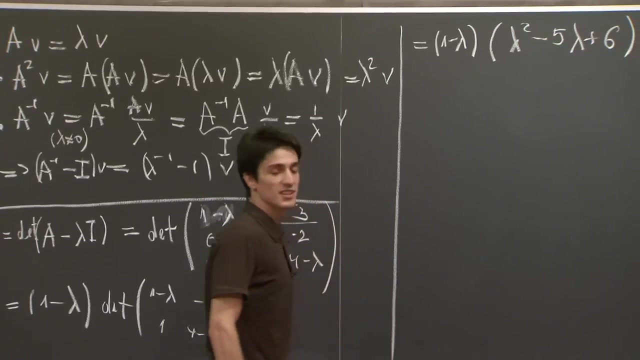 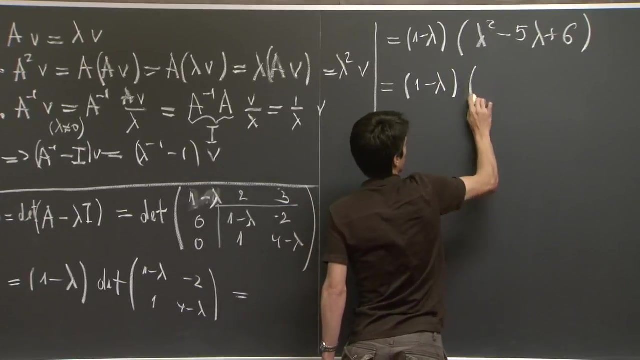 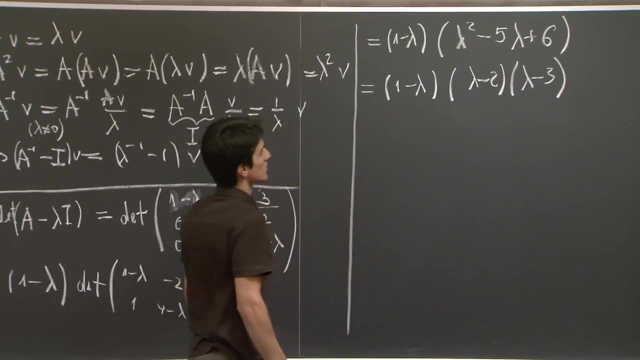 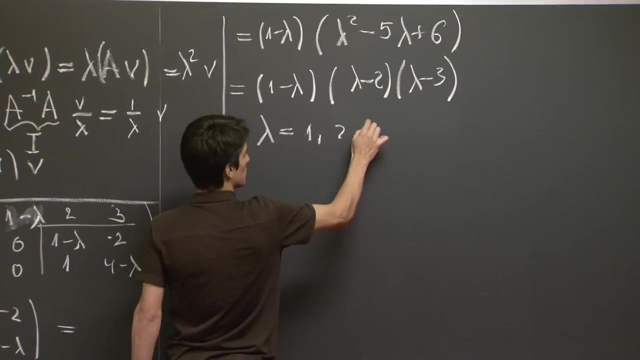 1 minus lambda. lambda squared minus 5, lambda plus 6,, which is a fairly familiar quadratic, And we can write it as a product of linear factors: It's lambda minus 2.. Lambda minus 2. 3. So the three eigenvalues of A are 1,, 2, and 3.. 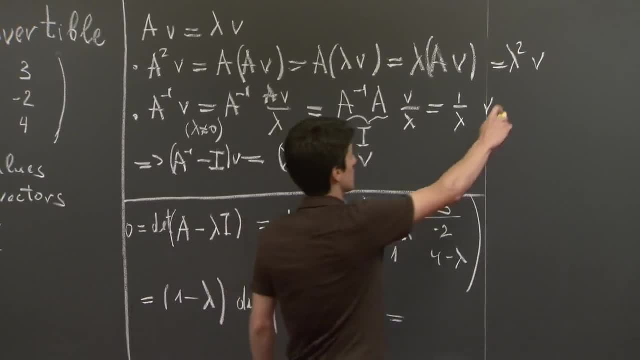 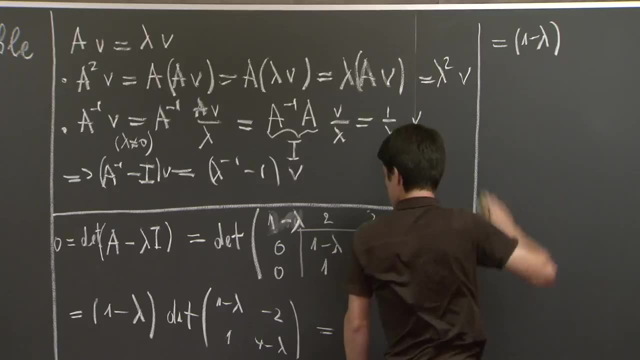 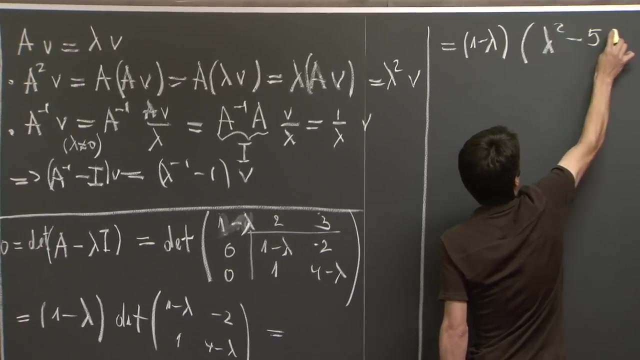 I'm going to take the second column, I'm going to take the third column, I'm going to take the fourth column And I'm going to take the computation up here: 1 minus lambda. Lambda squared minus 5. lambda plus 6.. 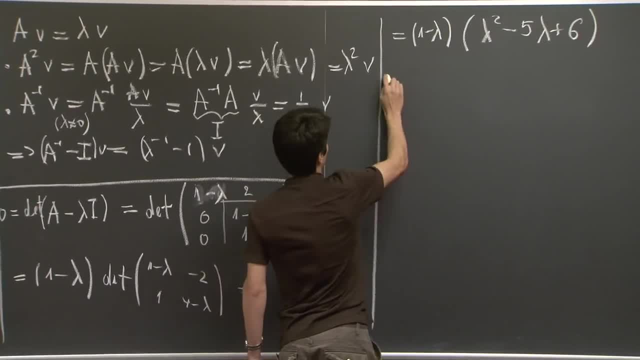 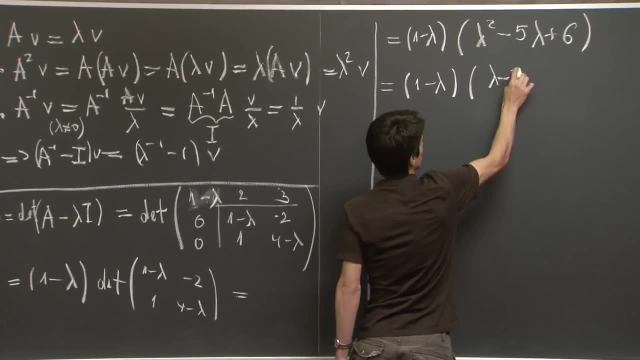 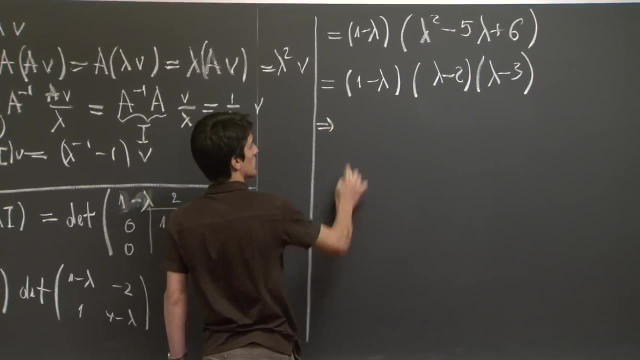 Which is a fairly familiar quadratic, And we can write it as a product of linear factors. It's lambda minus 2.. 1 minus lambda, Lambda minus 3.. So the three eigenvalues of A are 1,, 2, and 3.. 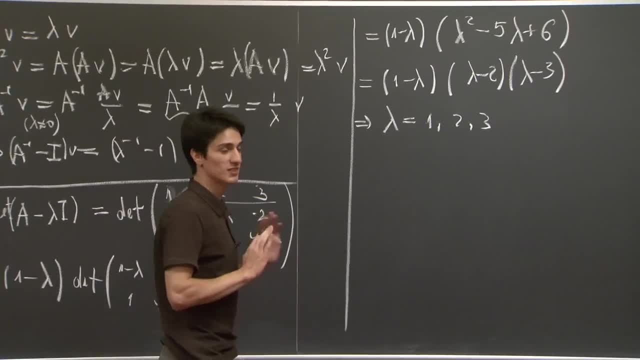 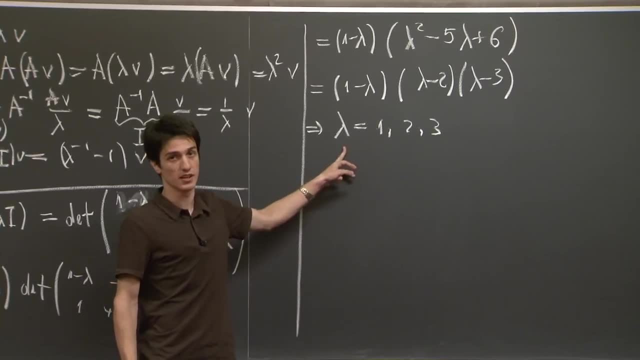 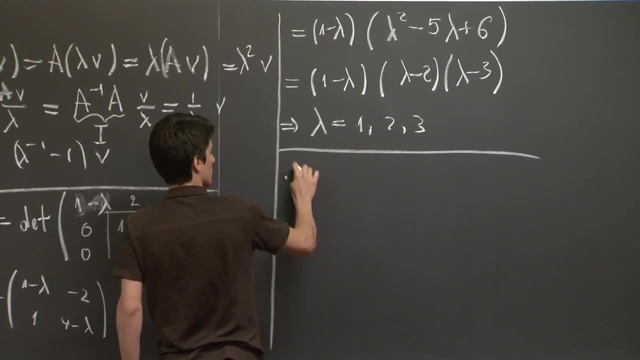 OK, So the first half of our problem is done. Now we just need to find what the eigenvectors associated with each of these eigenvalues are. How do we do that? Well, let's see, Say let's figure out what the eigenvector associated. 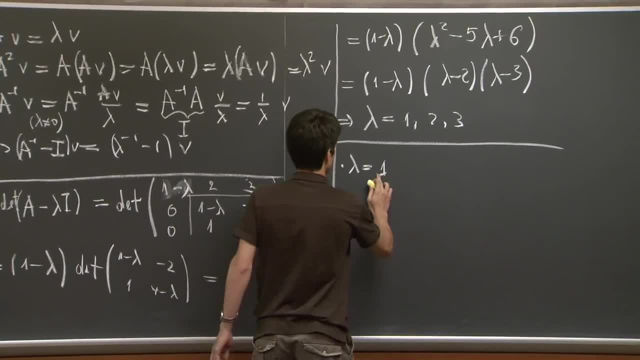 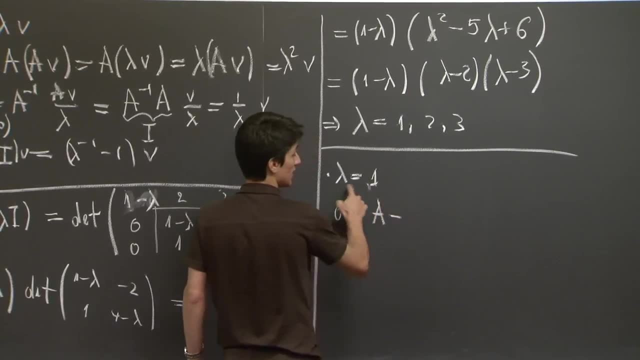 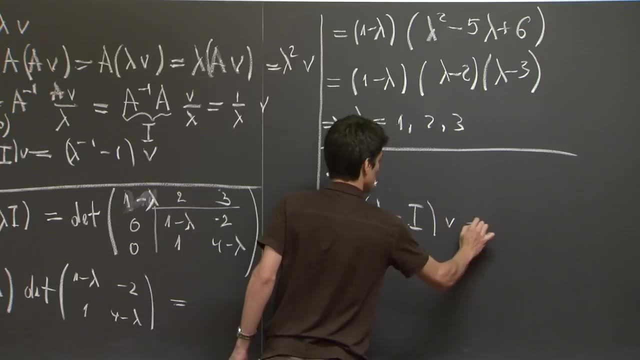 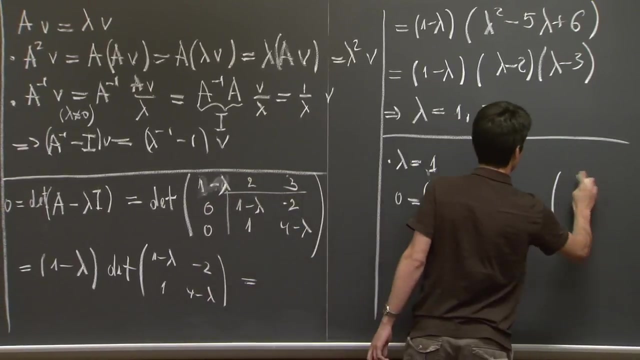 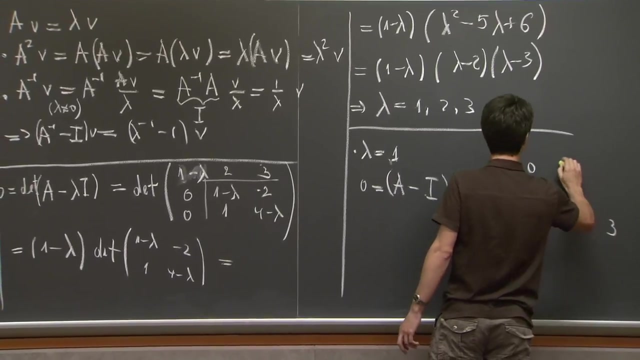 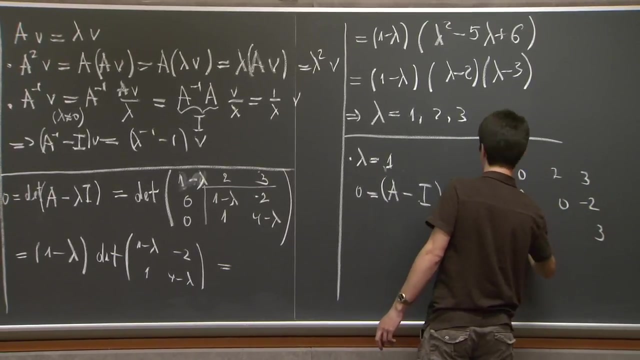 with lambda equals 1 is. So we know that the eigenvector needs to be in the null space of A minus lambda the identity. So A minus the identity V. So let me write this out: It's 0, 0, 3, 2, 3, 0, negative, 2, 0, 1.. 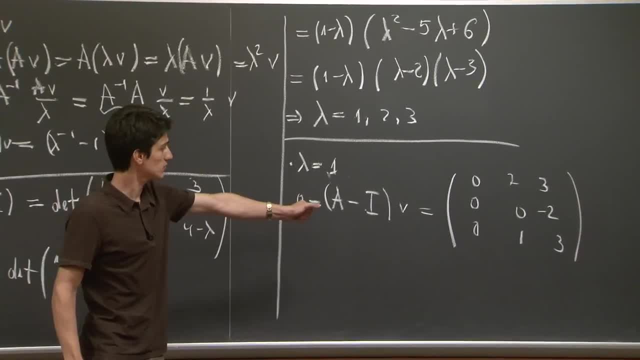 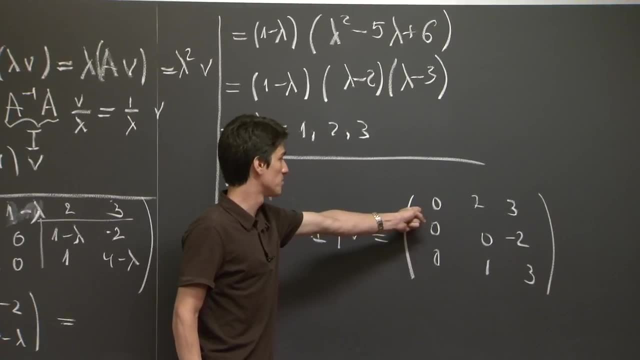 And we see that the first column is 0.. So well, the first, therefore, yeah, The first zero, The first zero, The first zero, The first variable will be our free variable if we want to solve this linear system of equations. 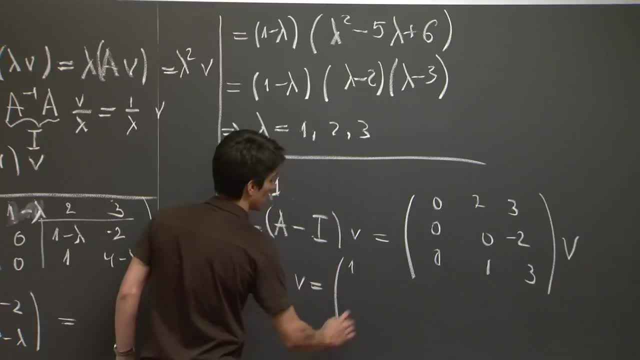 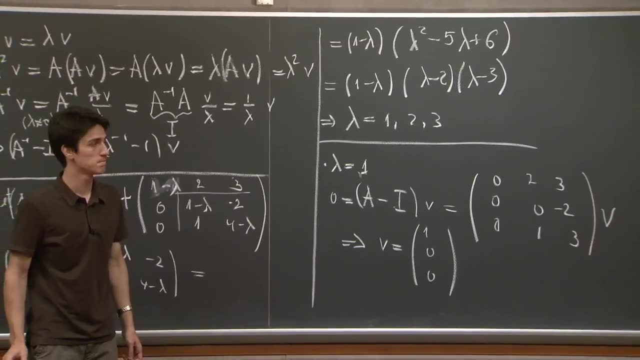 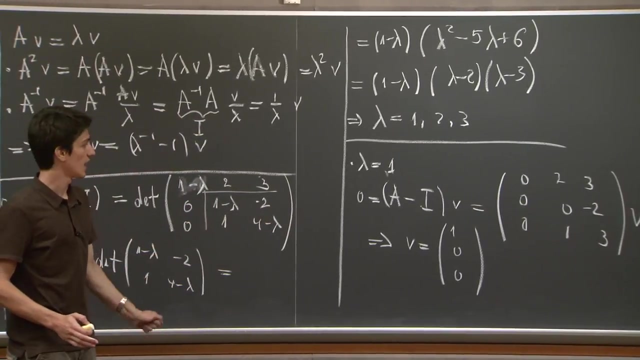 And we can just set it to 1.. And it's not hard to see that the other two entries should be 0. So we can do the same procedure with the other two eigenvalues And, yeah, we'll get an eigenvalue each. 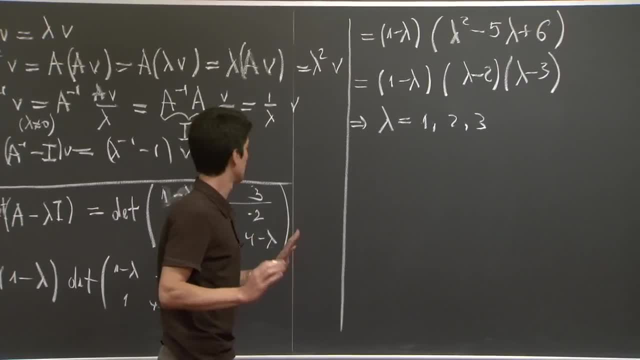 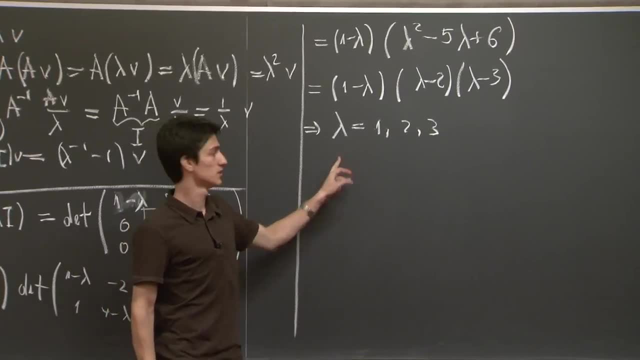 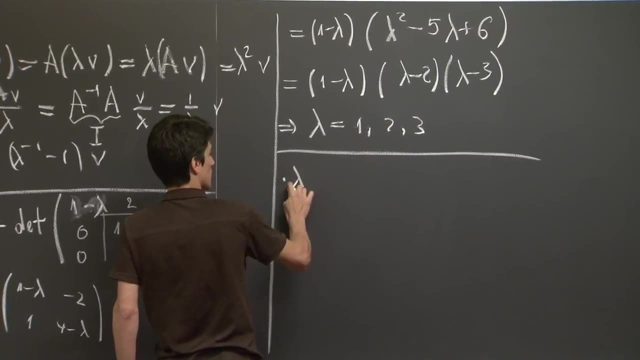 OK, so first half of our problem is done. Now we just need to find what the eigenvectors associated with each of these eigenvalues are. How do we do that? Well, let's figure out what the eigenvector associated with lambda equals 1 is. 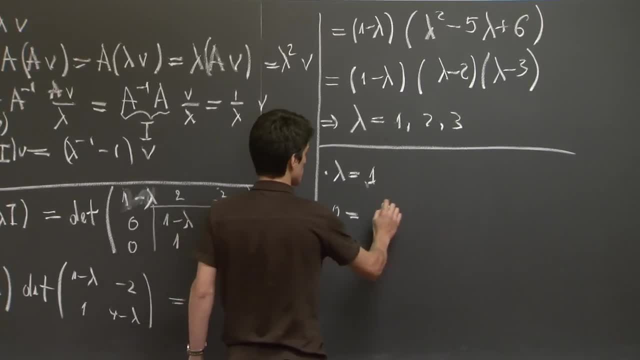 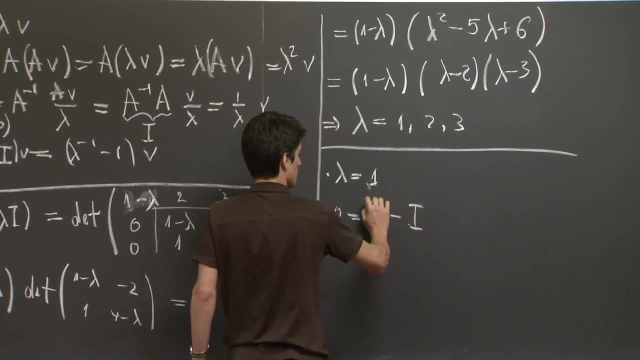 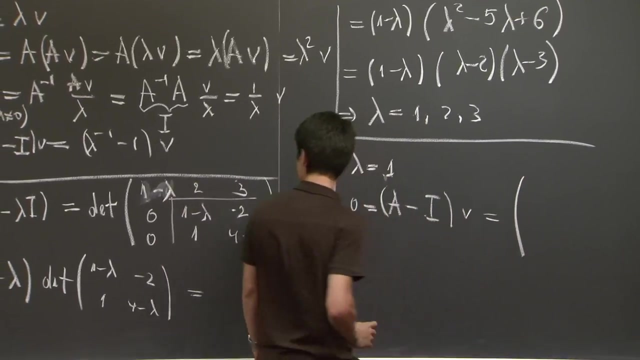 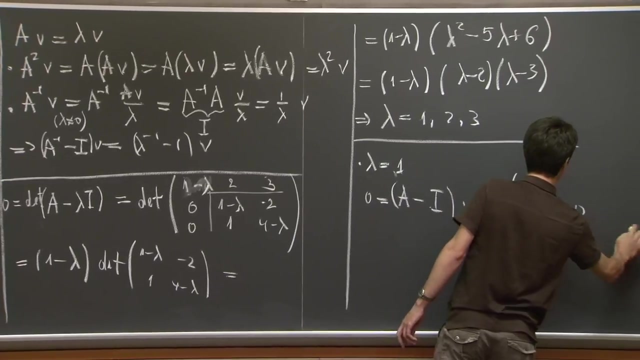 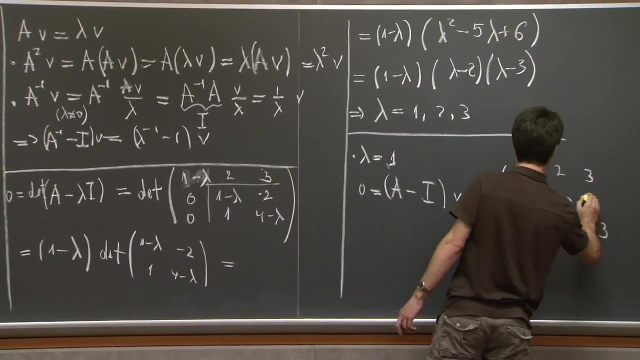 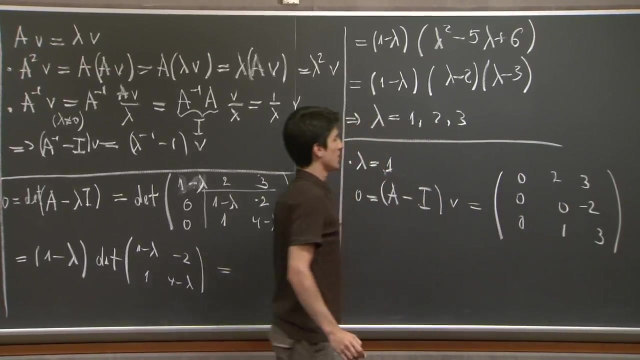 So we know that the eigenvector needs to be in the null space of A minus lambda the identity, So A minus the identity V. So let me write this out: It's 0, 0, 3, 2, 3, 0, negative 2, 0, 1.. 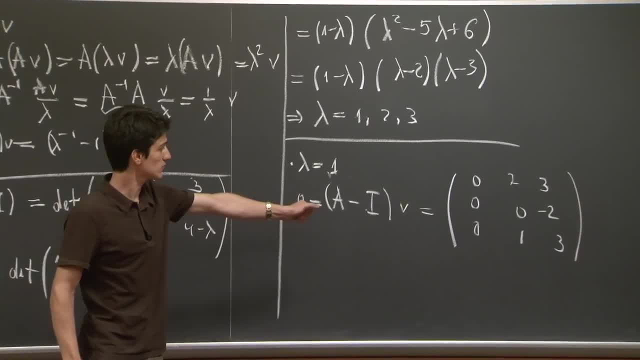 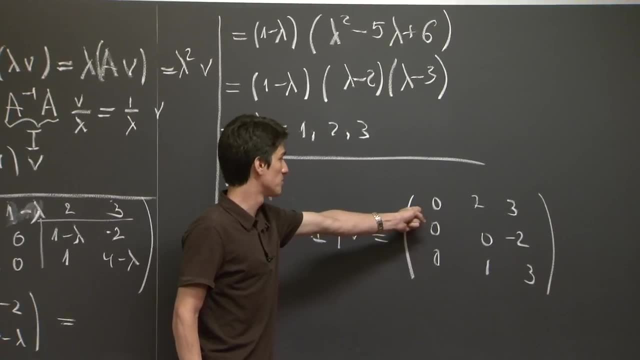 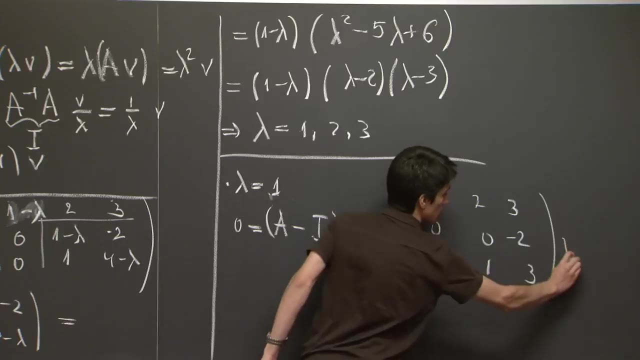 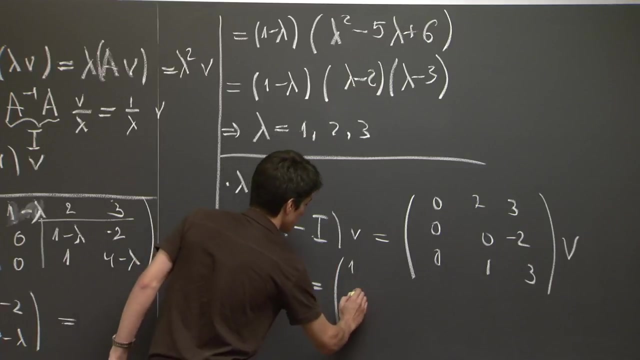 And we see that the first column is 0. So well, the first. Therefore, yeah, the first variable will be our free variable if we want to solve this linear system of equations, And we can just set it to 1.. And it's not hard to see that the other two entries should. 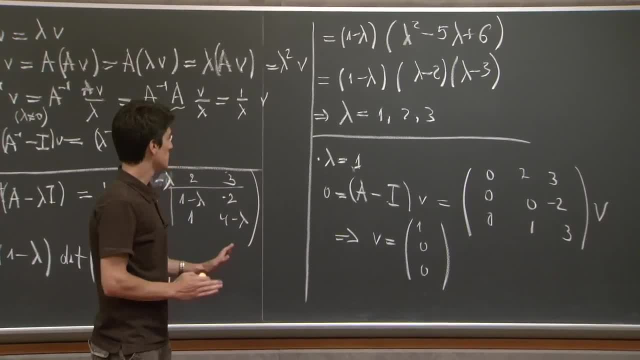 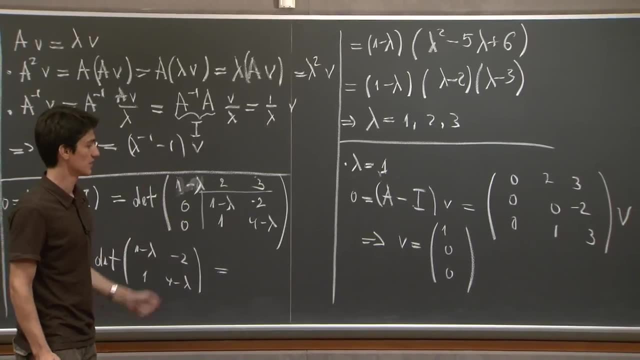 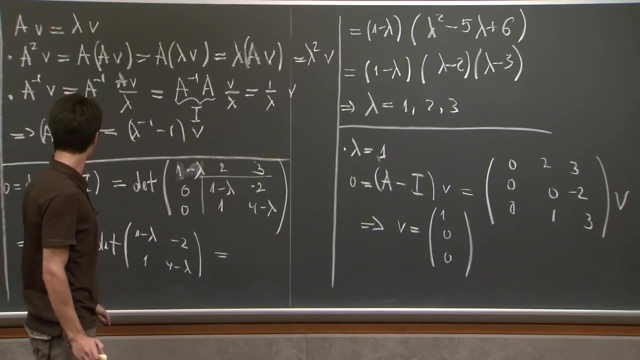 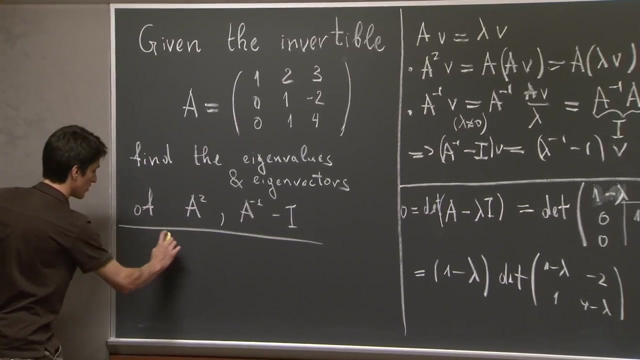 be 0. So we can do the same procedure with the other two eigenvalues And, yeah, We'll get an eigenvector for each eigenvalue. And in the end let me go back here. So I'm going to put our results in a little table. 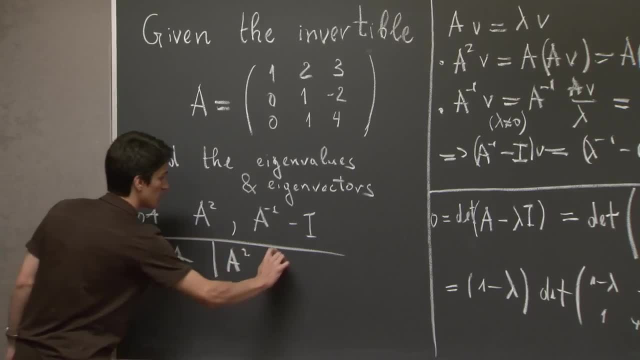 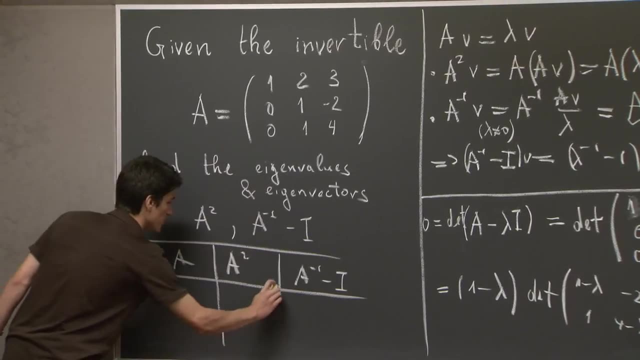 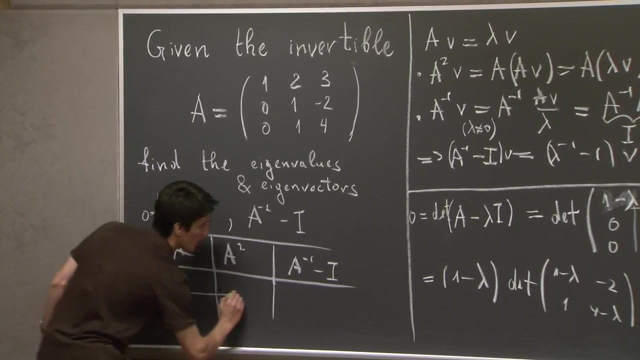 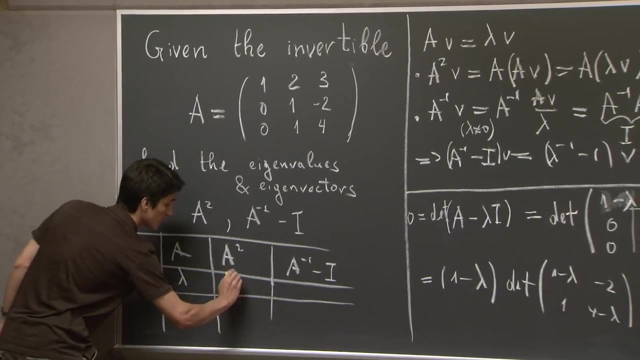 So A squared, and this is the identity. So, And the first row will be eigenvalues. So it's going to be: if lambda is an eigenvalue for A, then we saw that lambda squared will be the eigenvalue for A squared.